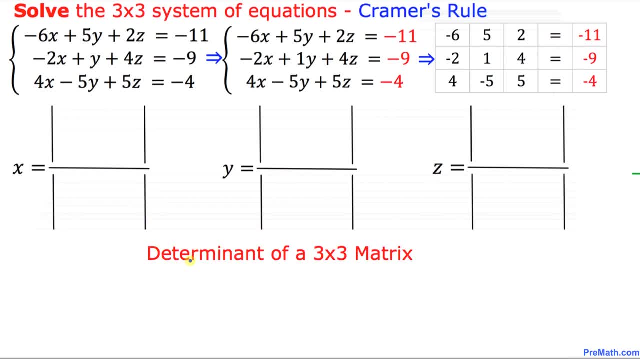 called the determinates of 3 by 3 matrix. Once again, these boxes are called the determinates. And now, in this next step, we have to start filling out these boxes, these determinates, And let's focus on these numbers on the left-hand side of these equal sign in this table. 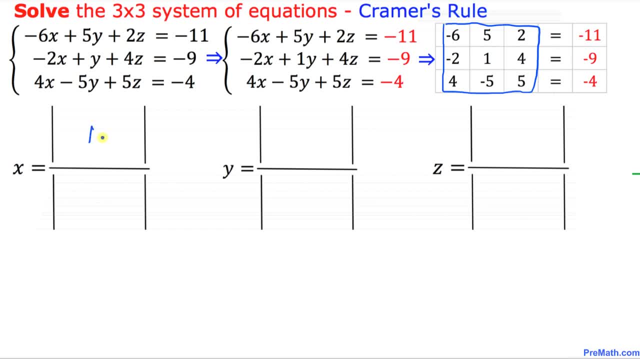 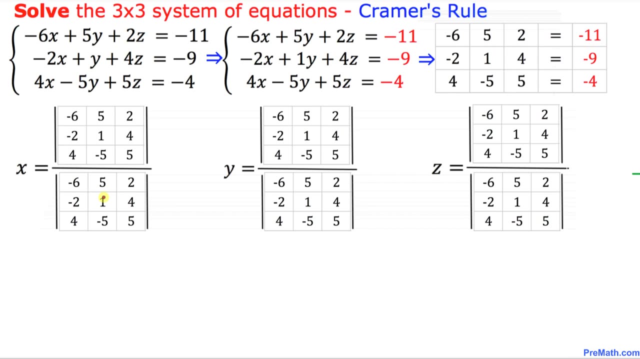 are going to fill in all these numbers, in all these determinants, all of them. we are going to fill them out. and here we have nicely filled out these numbers in each of every of these boxes. and now let's focus on these numbers. this column on the right hand side with red numbers: 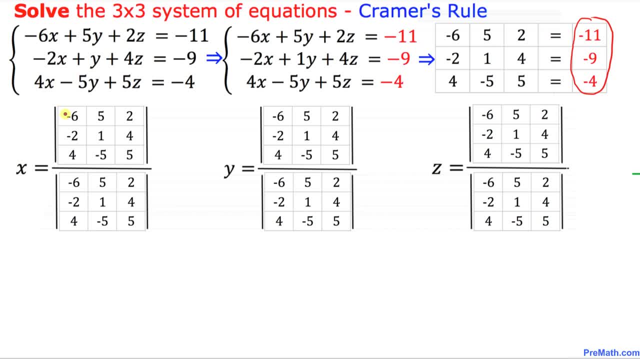 these numbers are going to go for x variable, that's going to go for left, the very first column. as we go along they are going to shift. for y they go in the second column, in the middle, and for z they're going to go all the way to the right hand side, to the third column. and here is 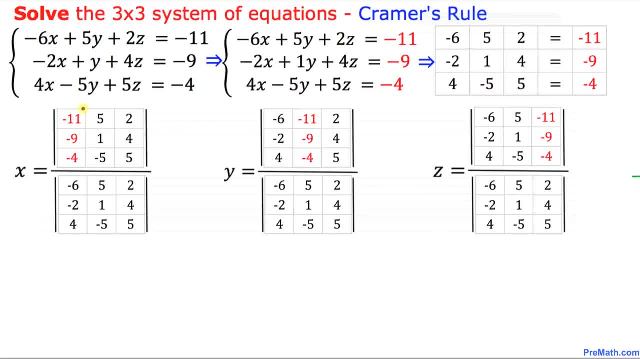 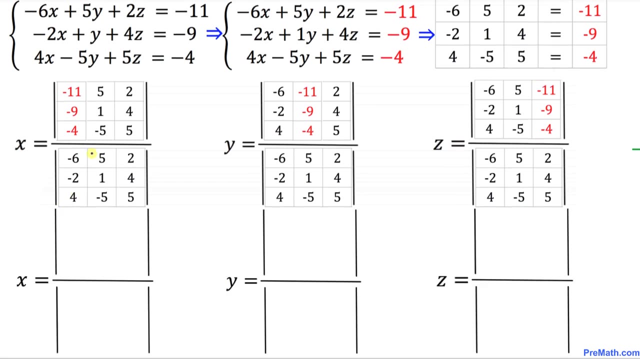 our final product. as you can see, these red numbers showed up for x in the very first column, for y in the second column and for z in the third column. and now i can nicely filled out these numbers by myself, let's go ahead and start filling out. so the first box, first determinant, could be written as negative 11. negative 9. 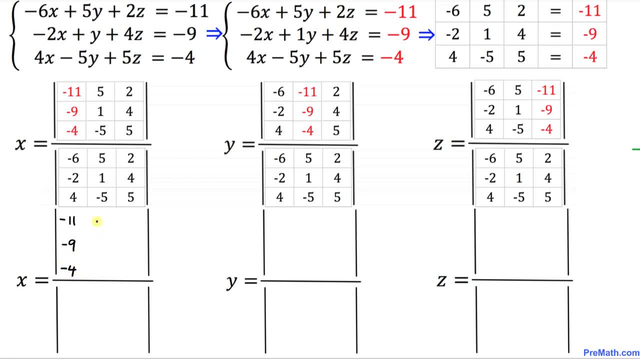 negative, 4, and then 5, 1, negative, 5, and on the right hand side it's going to be a 2 4, 5, and we start filling out negative 6, negative 2, 4, negative 11, negative 9, negative 4, 2, 4, 5. and here we have filled out all these determinants, as you can see. and now, in this next 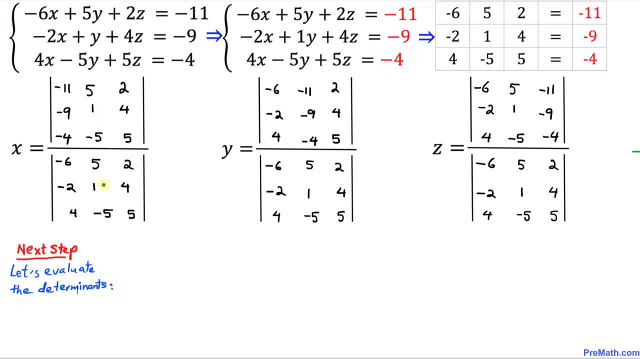 step. we are going to evaluate each and every determinants as you can see, one at a time. let's start off with finding the value of this bottom determinant, and here i have copied down this determinant right up here and now let me show you the easiest possible. 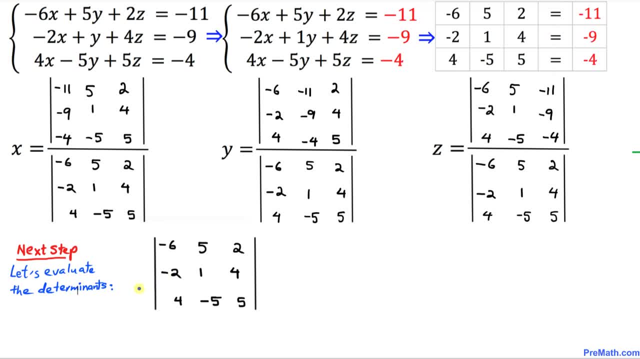 way to find the value of this determinant. the very first thing is we are going to draw this horizontal line right above this last, this row, and now we are going to crisscross. let's multiply negative 6 times 1. it is negative 6. then you put a minus sign. 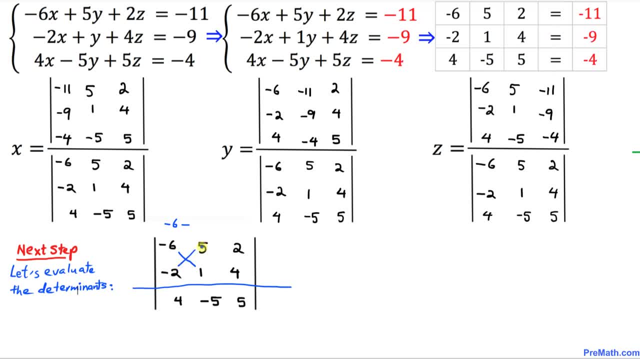 and then a sign. let's cross. multiply the other way around: five times negative two is negative 10. so this makes negative six, negative and negative to become positive 10. that's gonna give us positive four. this positive four goes in the opposite side, opposite direction. let's repeat. 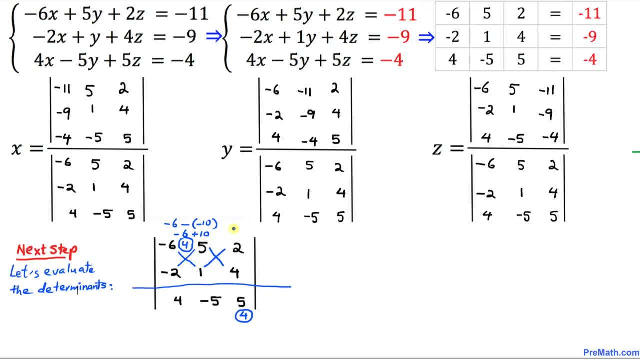 this process with next two columns crisscross four times five is 20, and then we put a minus sign. and then we repeat this process with next two columns: crisscross four times five is 20, and then we put a mind sign, minus sign, 2 times 1 is 2, 20 minus 2 is 18, so 18 is going to go in this opposite side. 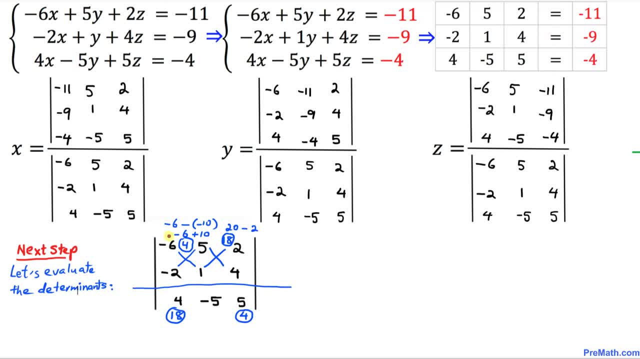 all right. and then, finally, we're going to look at this very first column. we're going to copy and paste right on this side: negative 6,, negative 2, let's crisscross once again: cross, multiply 2 times. negative 2 is negative 4, then we put a minus sign. cross, multiply this way. 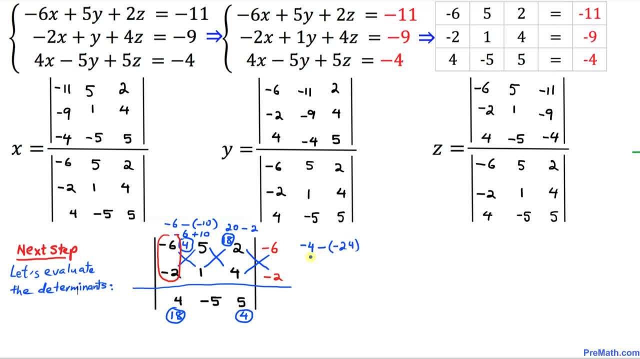 that's going to be negative 24, so this becomes negative 4 plus 24, that is going to give us positive 20, so this positive 20 is going to go in the middle. let's go ahead, and now. first we're going to multiply these. 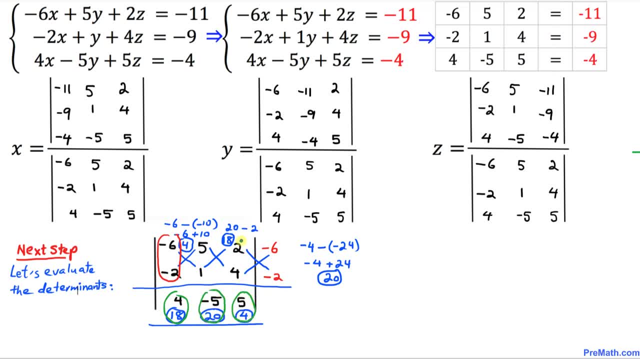 numbers, numbers, and then we're gonna add them up. let's see: 4 times 18 is 72, and then 5 times 20, with a minus sign, is gonna be a negative 100, and then plus 20, 5 times 4 is 20, and if you look at this, 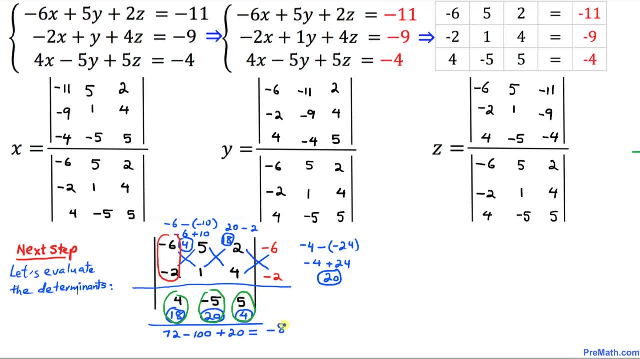 thing that is gonna give us negative 8. all right, so this is the value of this bottom determinant, which is negative 8. as you can see that these three, all these three determinants are same, so they're gonna have same value. I'm gonna write down over here: negative 8 and negative 8 over here. 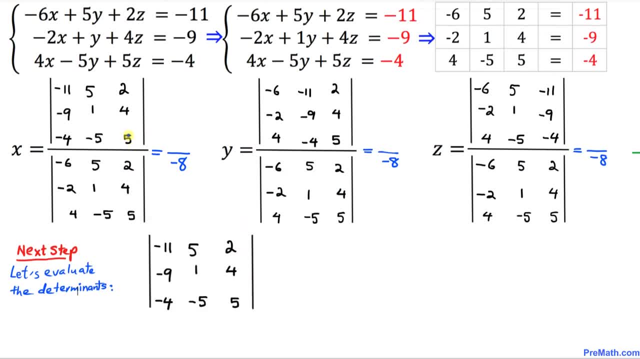 as well. and now we are going to evaluate this top part of x, which I have just copied down over here once again. let's go ahead and draw the horizontal line right above this last row. let's crisscross, multiply, cross, multiply first. this way: negative 11 times 1 is a negative 11. 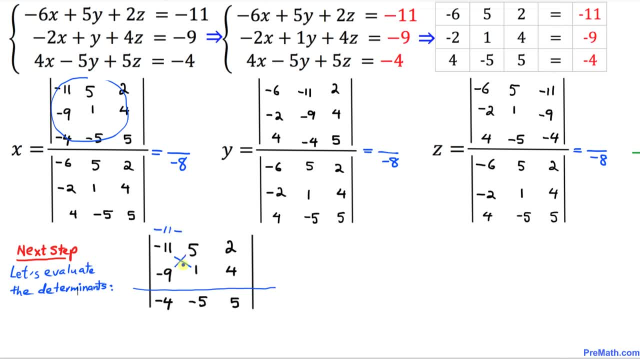 put a minus sign and then 5 times negative. 9 is negative 45. so that is going to give us a negative 11. negative a negative becomes positive 45 and that is gonna give us 34. So this 34 is going to go in this opposite side over here. all right, now let's. 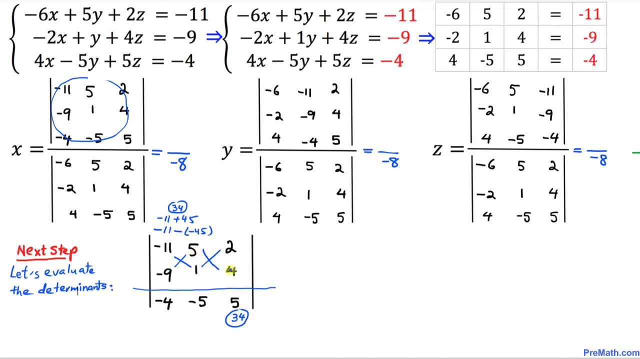 crisscross the next two columns over here. 5 times 4 is 20 For a minus sign. 2 times 1 is 2,. 20 minus 2 is 18, 18 is going to go in the opposite side, over here. 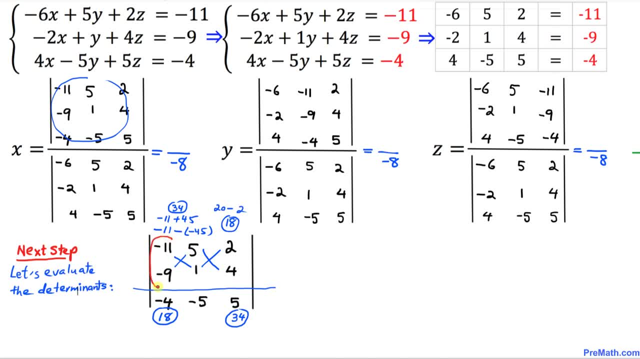 Now the next step is we are going to copy this very first column, negative 11 and negative 9, and paste on this side. as you can see, Let's repeat the process again. We are going to criss-cross 2 times. negative 9 is negative 18, let's put a minus sign. 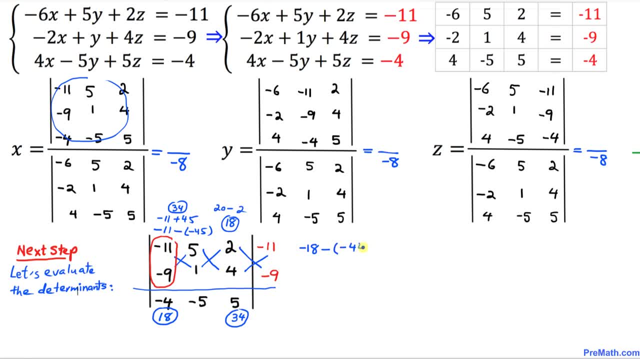 negative 11 times 4 is negative 44,. let's simplify: negative 18 plus 44 is going to give us positive 26.. This positive 26 goes in the middle. Now the last step is just Multiply these numbers first, and then we are going to add them up. 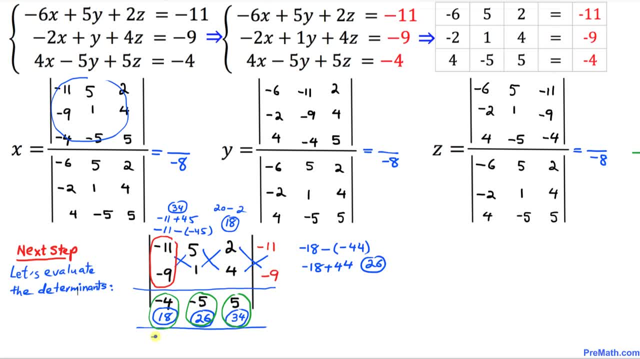 Let's multiply them first. That is going to be negative 72 minus 130 and plus 170, and if we simplify these numbers, we are going to get negative 32.. Okay, So this negative 32 is going to go on the top over here. 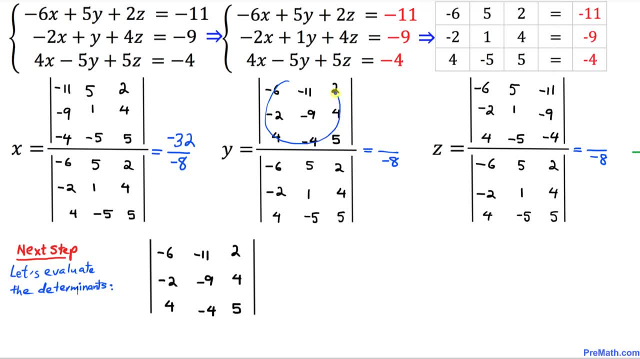 And now we are going to evaluate this determinant on the top and which I have copied down right up here. The very first thing is draw the horizontal line right up here and then let's criss-cross. Okay, So negative 6 times negative, 9 is going to be 32.. 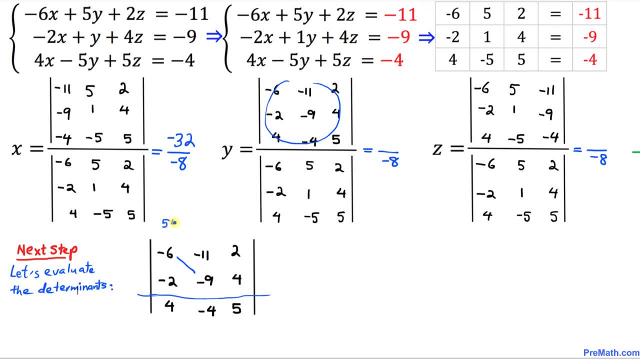 Okay, So this is going to be positive 54, then we put a minus sign and we multiply this way, So that's going to give us positive 22.. So that is going to give us 32.. As you can see, this one, when you subtract this, 32 is going to go in this opposite side. 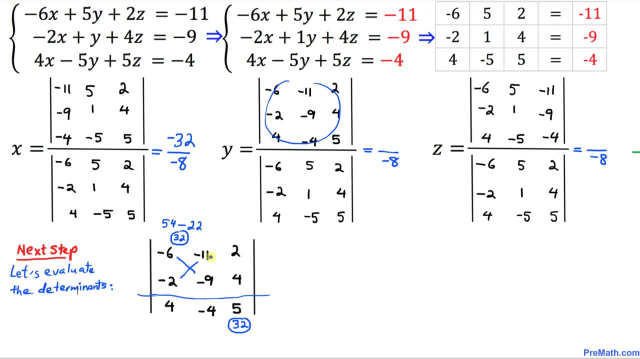 as you can see, Let's criss-cross the next two columns. Negative 11 times 32.. Negative 11 times 4 is negative 44. Then we put a minus sign 2 times negative: 9 is negative 18.. 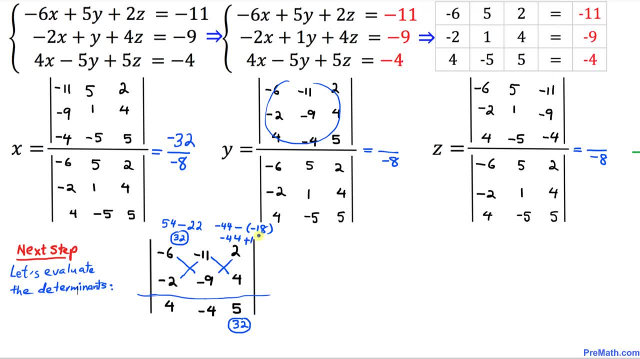 So negative 44 plus 18, and if we simplify that one, that is going to give us negative 26.. All right, This negative 26 is going to go in this opposite side. Okay, So this is going to give us negative 26.. 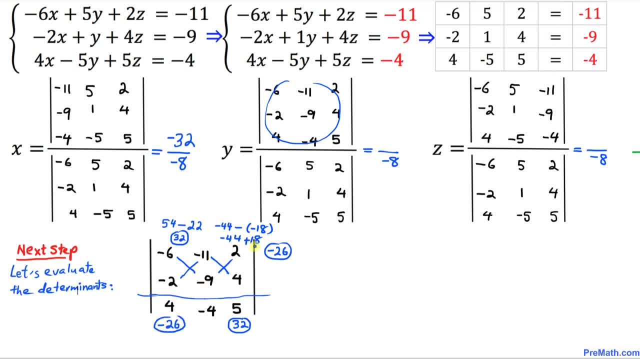 All right, So negative 26 is going to go in this opposite side, And now we are, our next step is: we are going to copy this number, this column, Negative 6 and negative 2 over here and let's criss-cross once again. 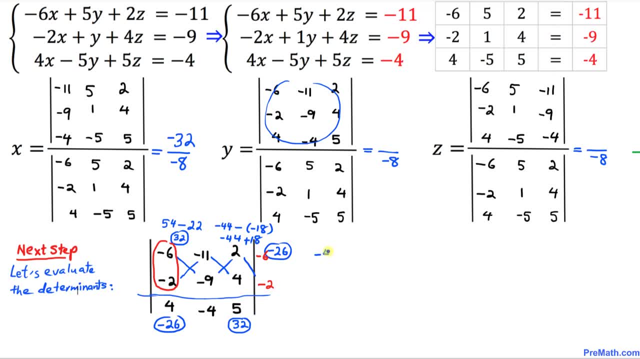 We're going to multiply 2 times negative. 2 is negative 4, put a minus sign: Negative 6 times 2 is negative 24.. So that's going to become negative 4 plus 24 is going to be positive 20.. 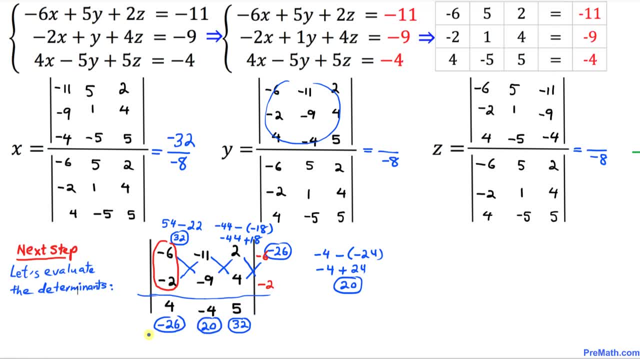 That is going to go in the middle over here. Let's simplify these one: First we are going to multiply these numbers and then we are going to add them. So let's multiply them first. So that is going to give us negative 104.. 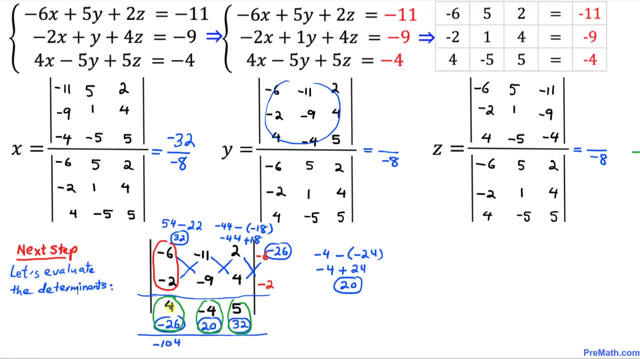 When we multiply, So that is going to give us negative 104.. Okay, So we are going to multiply 4 times negative 26.. And then that is going to give us negative 4 times 20 is negative 80.. And then plus 5 times 32 is 160.. 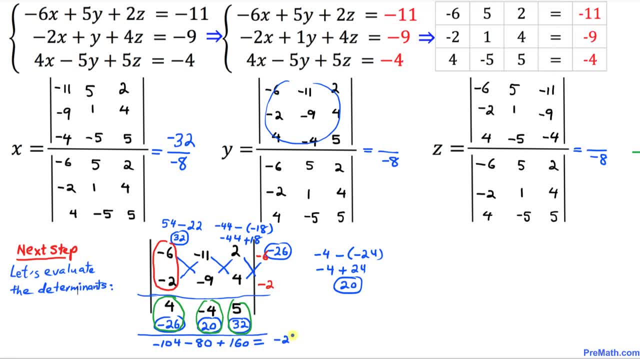 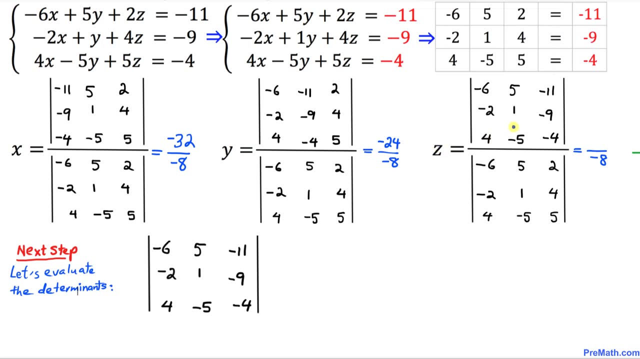 Let's simplify these. one That's going to give us negative 24.. So that means this number, the value of this top determinant for y, 10 to the power of 5, turns out to be negative 24.. And now we are going to find the value of this determinant for z on the top, which I 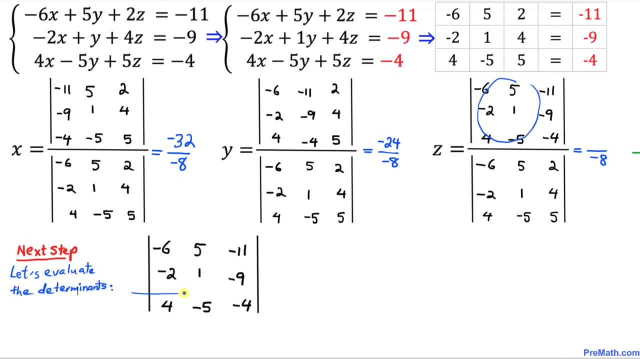 have just copied down Once again. the very first step is draw this horizontal line first, and now start cross, multiplying, crisscross: Negative 6 times 1 is negative 6, put a minus sign. Negative 2 times 5 is negative 10.. 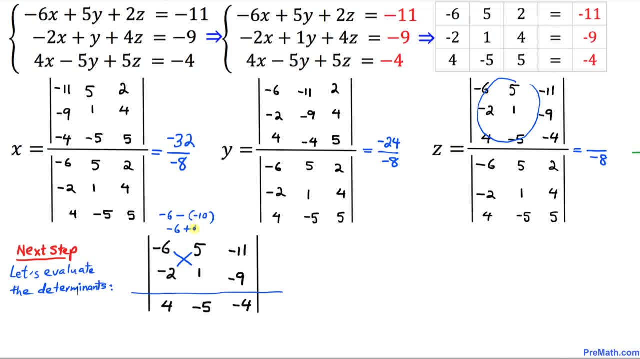 Okay, So that becomes a negative. 6 plus 10 is positive 4.. So positive 4 is going to go in the opposite side. And now let's crisscross these two numbers: Negative 5, 9 times 5 is negative 45.. 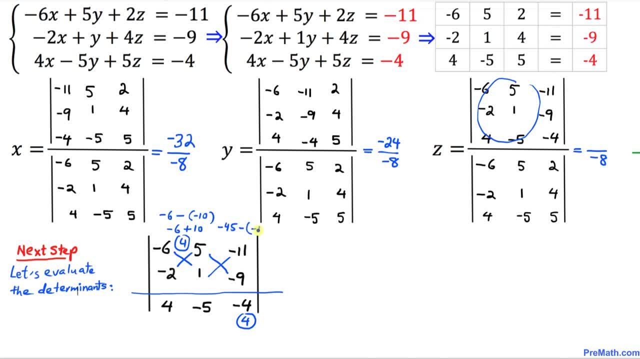 And then minus 1 times negative 11 is negative 11.. So negative 45 plus 11 is going to be negative 32.. Okay, So negative 4 is going to go in the opposite side. and finally, we are going to copy this: 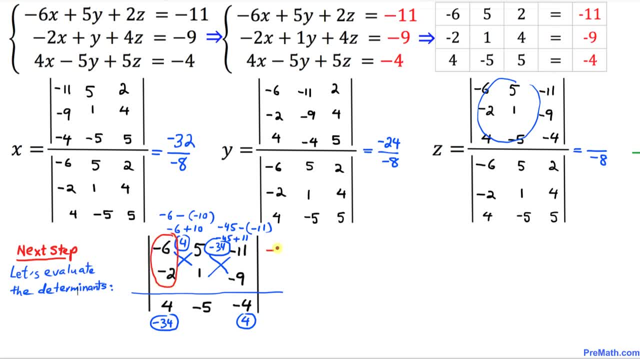 very first column on the left-hand side and paste it on this right-hand side And let's crisscross once again. Negative 11 times negative: 2 is positive 22,. then put a minus sign. Negative 6 times negative: 9 is positive 54.. 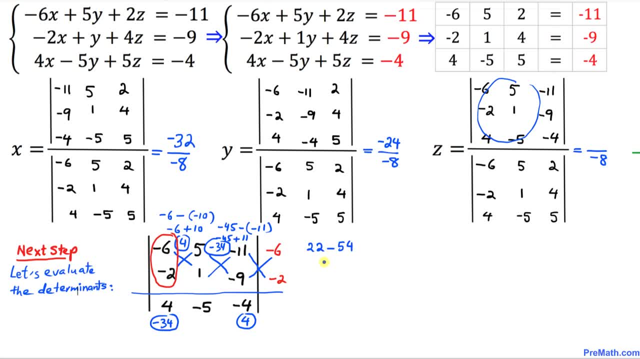 Okay, And that is going to give us negative 32, which is going to go in the middle. And now our final step is: let's simplify these. First, we are going to multiply these numbers first, and then we are going to add them. 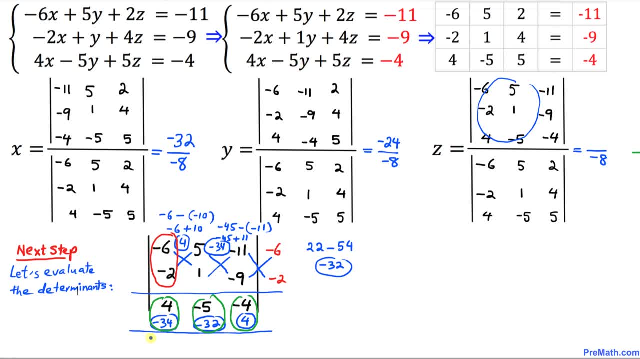 So 4 times negative, 34 is going to be negative 130. Okay, And that is going to be 6, plus that is going to be 160, and then minus 16. And if we simplify these numbers, we are going to get 8.. 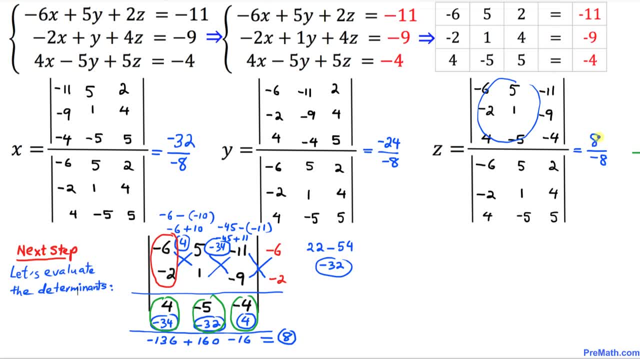 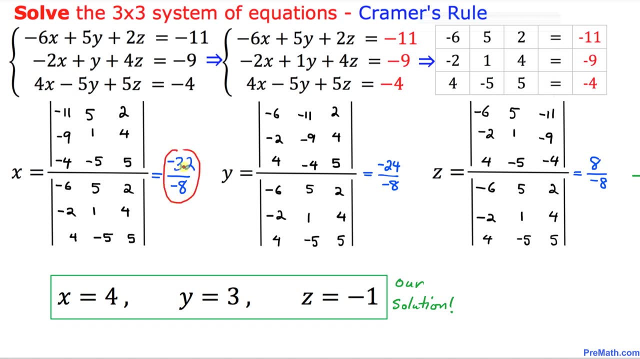 So that means this value for this z variable is going to be 8 on the top determinant. Okay, Okay, If we simplify, if we reduce this x value- negative 32 over negative 8, we are going to get x equal to positive 4.. 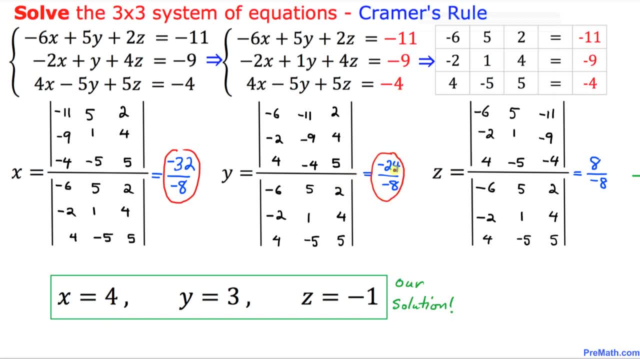 And likewise for y variables. if we reduce these one negative 24 over negative 8, give us y equal to 3.. And finally, for z variable: 8 over negative 8 is going to be negative 1. And that is going to be 4.. 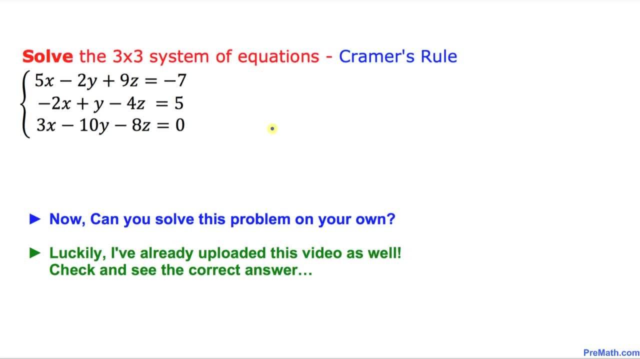 Okay, That is our answer And here is your assignment. Can you do this problem on your own? You can take your time. You can pause the video. Luckily, I have already uploaded this video as well. Please go ahead and check it out and see the correct answer.